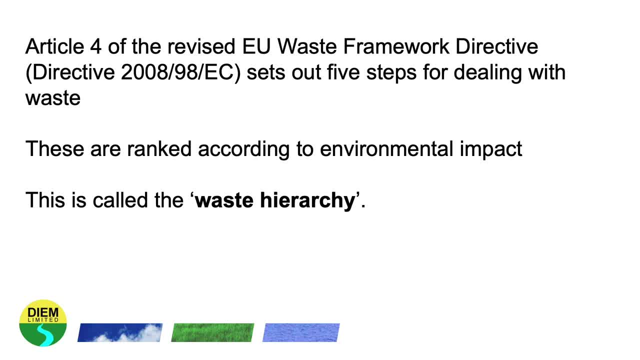 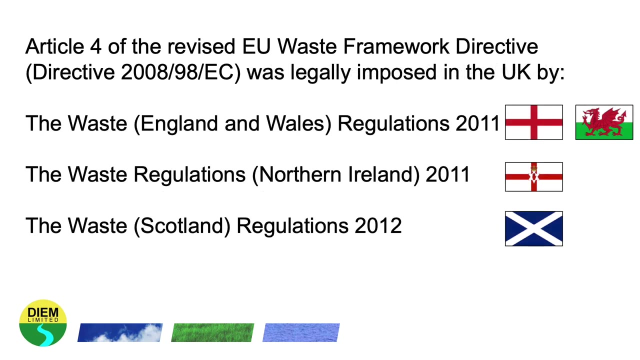 The five steps of the waste hierarchy came from the EU Waste Framework Directive and these five steps are ranked according to their environmental impact. and this is the waste hierarchy In the United Kingdom. it's been imposed as legislation in all four countries and it is a legal requirement across the United Kingdom. 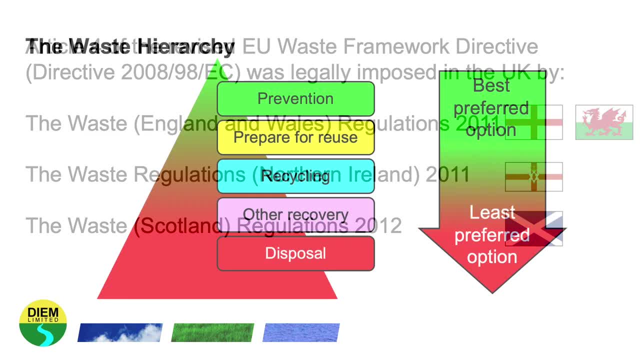 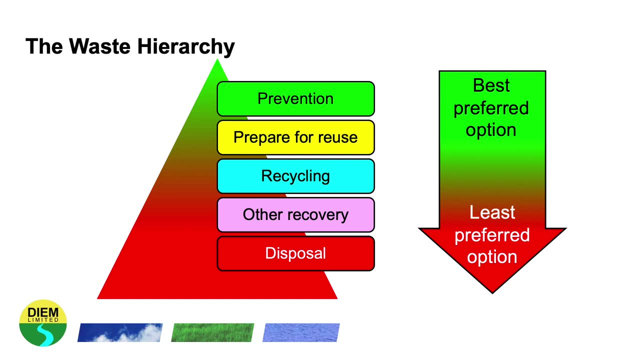 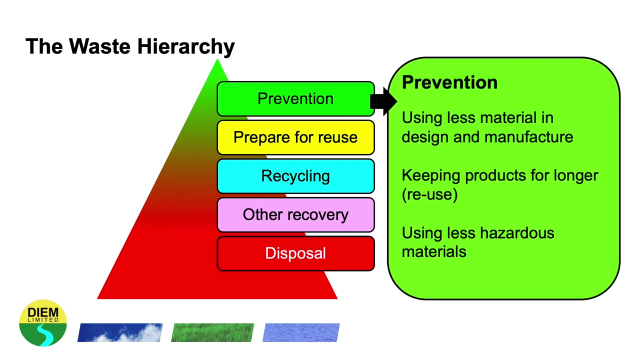 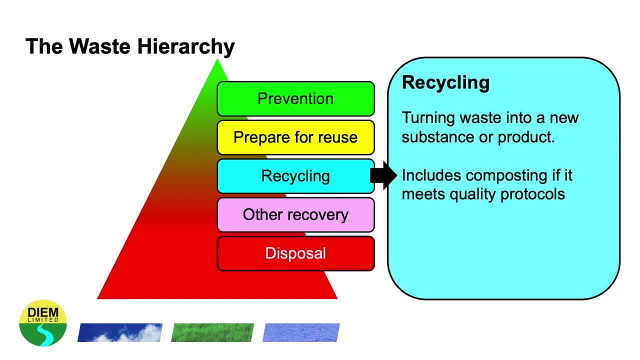 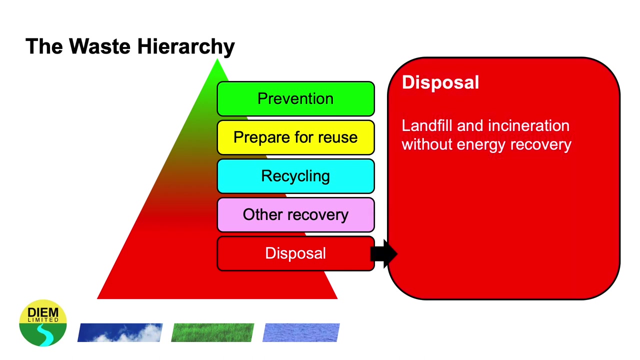 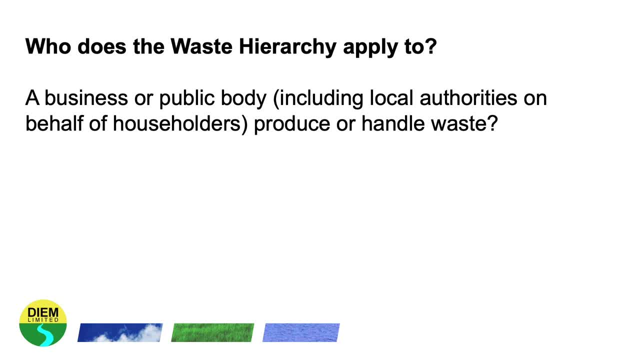 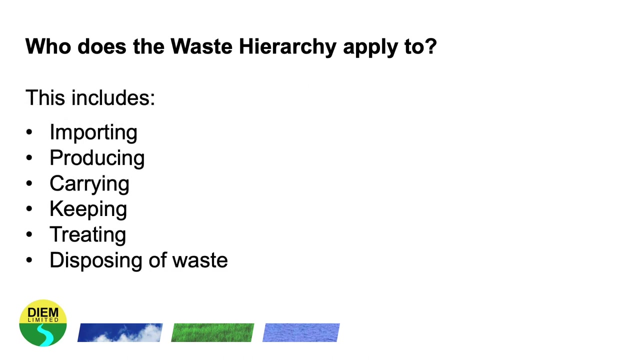 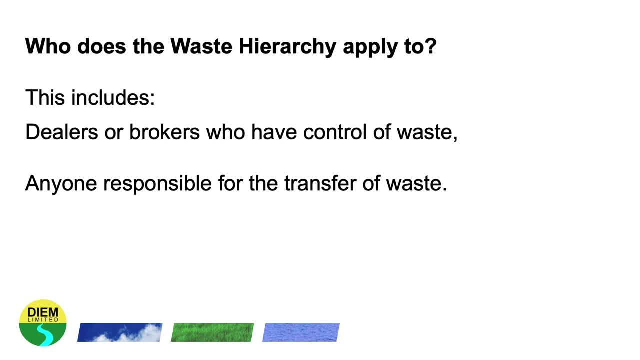 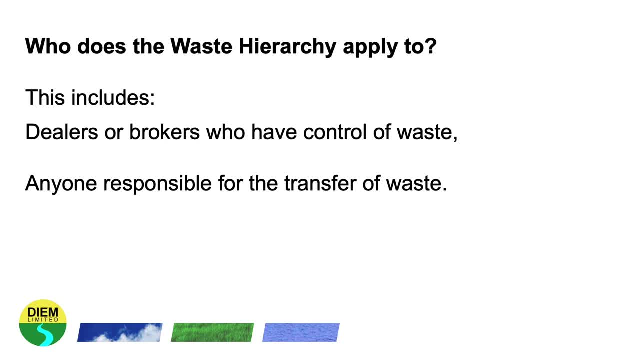 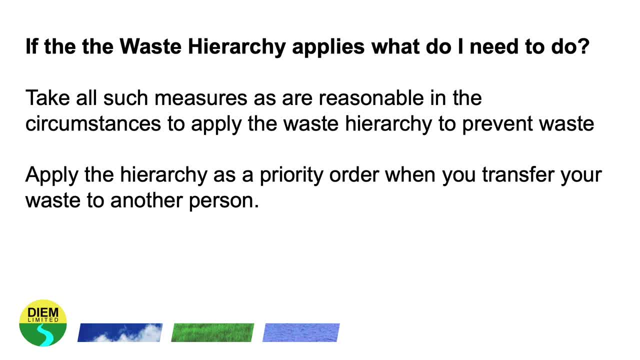 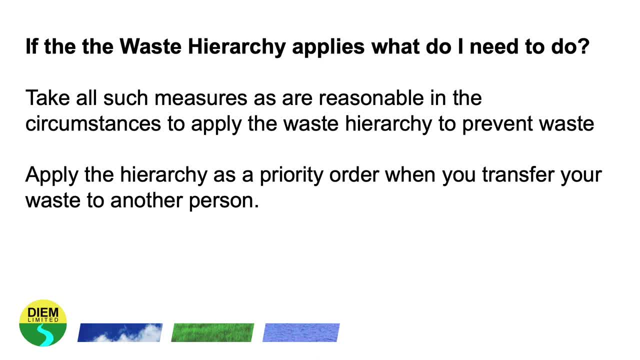